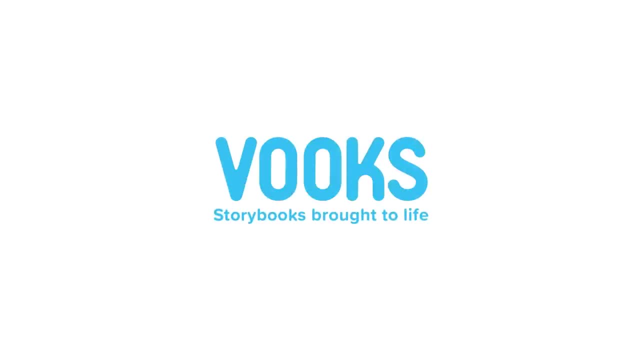 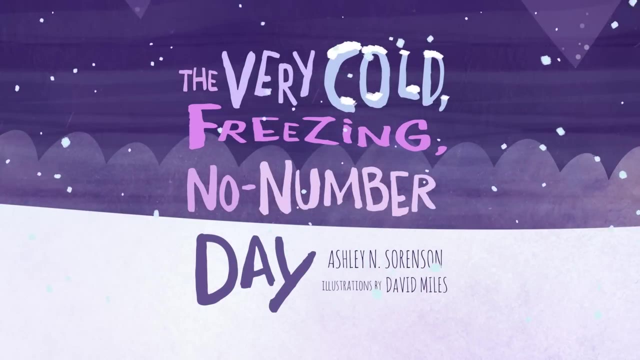 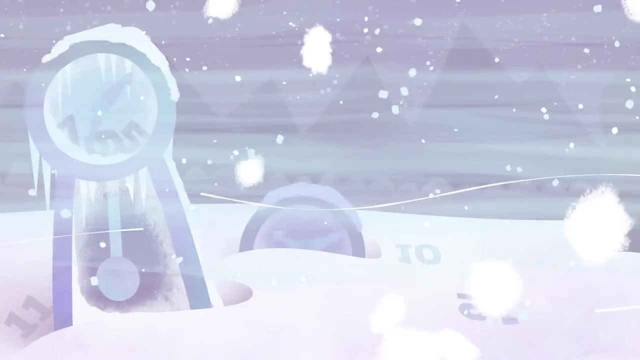 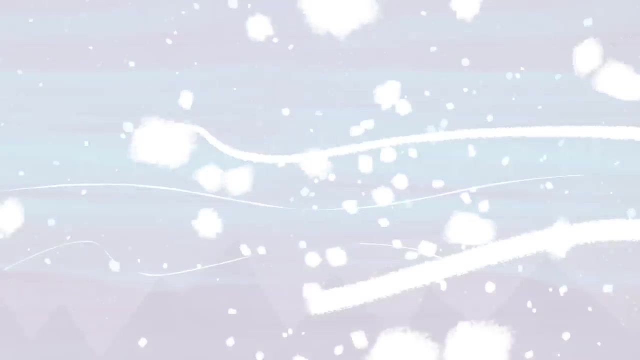 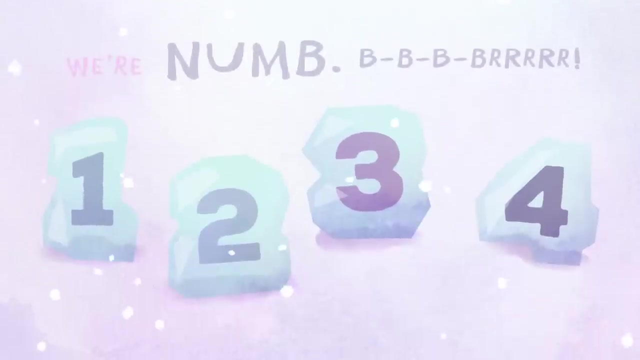 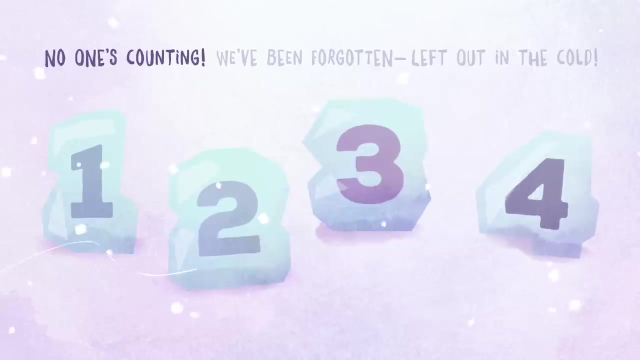 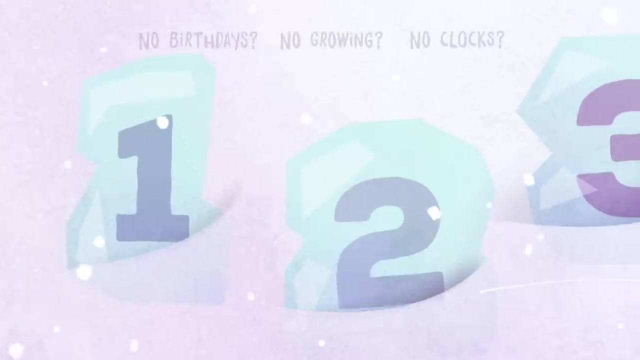 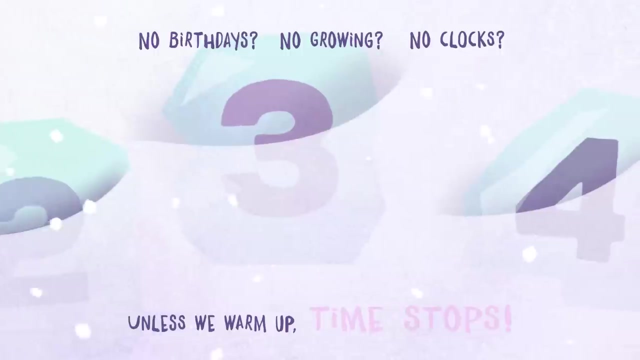 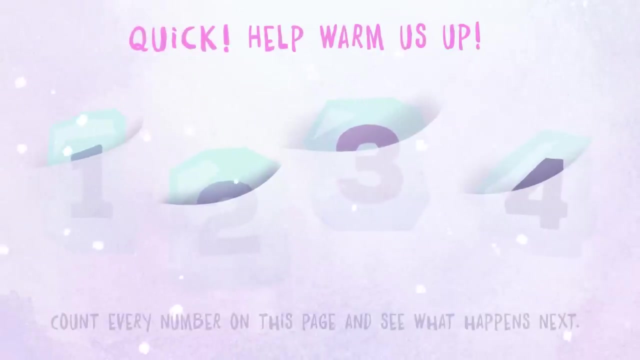 The very cold, freezing, no-number day. No one's counting. We've been forgotten, Left out in the cold. No birthdays, No growing, No clocks. Unless we warm up, time stops. Quick help, warm us up. Count every number on this page and see what happens next. 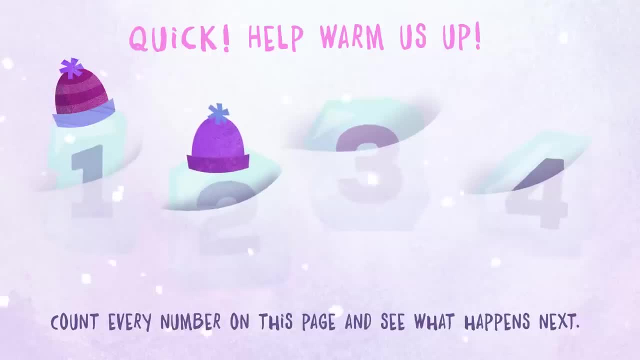 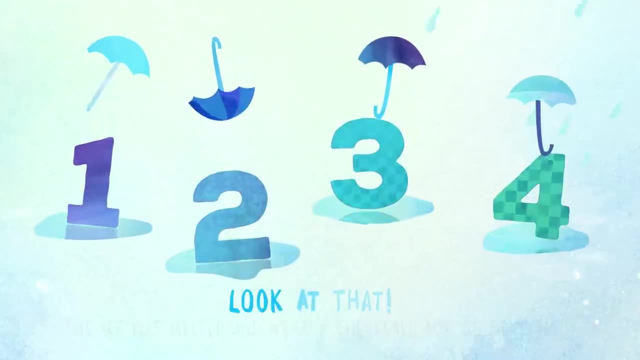 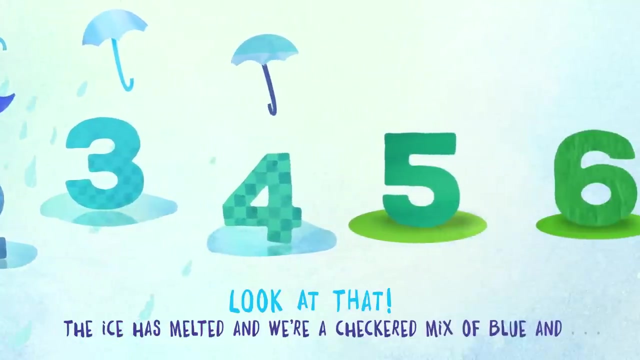 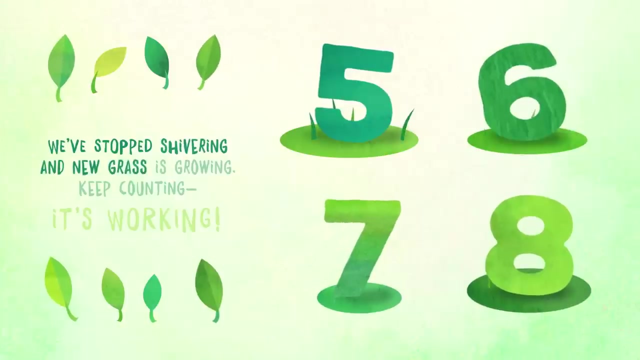 One, Two, Three, Four. Look at that. The ice has melted and we're a checkered mix of blue and Green. We've stopped shivering and new green. The grass is growing. Keep counting, It's working. 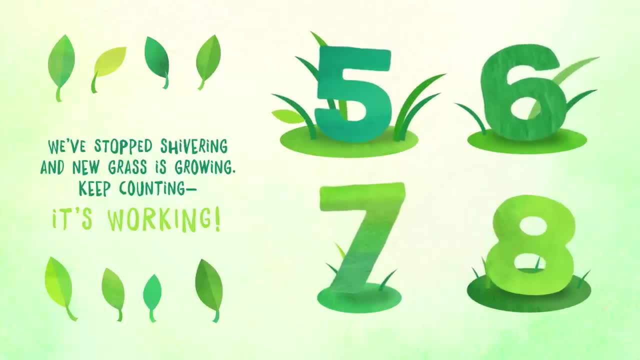 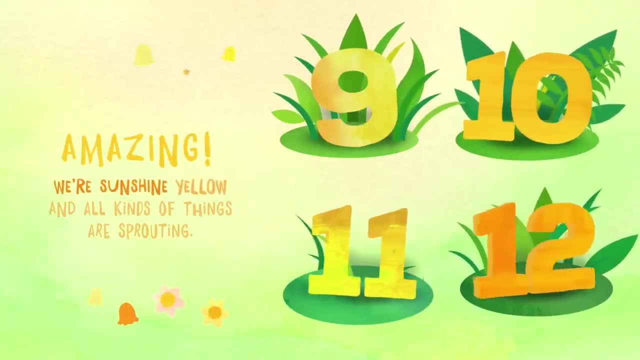 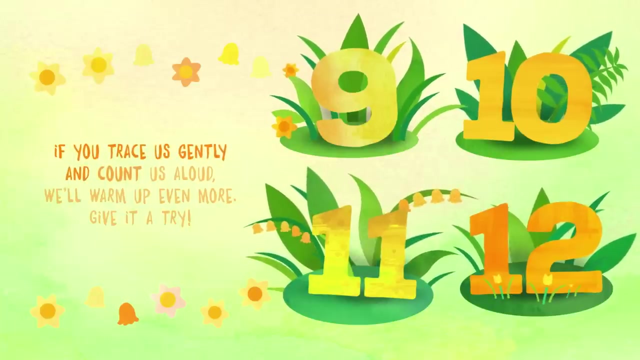 Five, Six, Seven, Eight, Amazing. We're sunshine, yellow and all kinds of things are sprouting. If you trace us gently and count us aloud, we'll warm up even more. Give it a try. Nine, Ten, Eleven, Twelve. 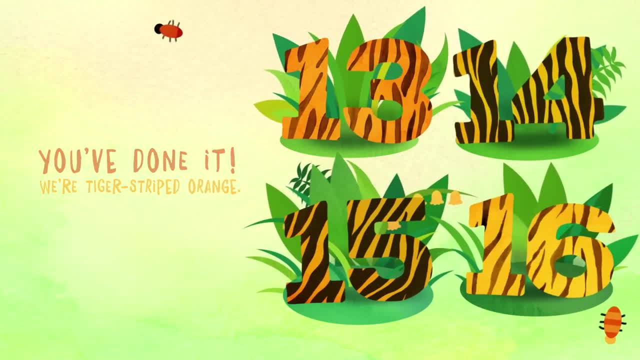 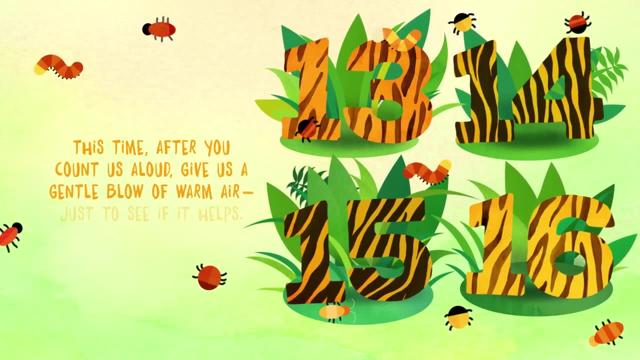 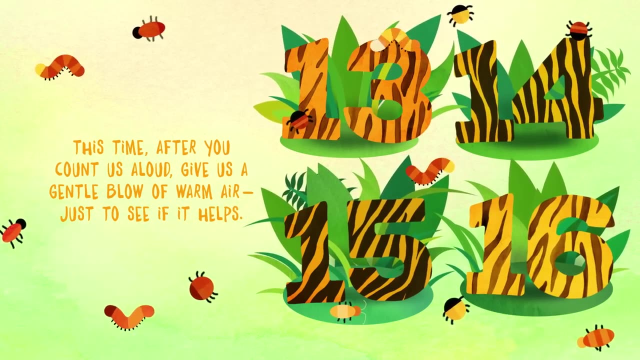 You've done it. We're tiger-striped orange This time, after you count us aloud, give us a gentle blow of warm air. Phew, Just to see if it helps. Thirteen, Fourteen, Fifteen, Sixteen. 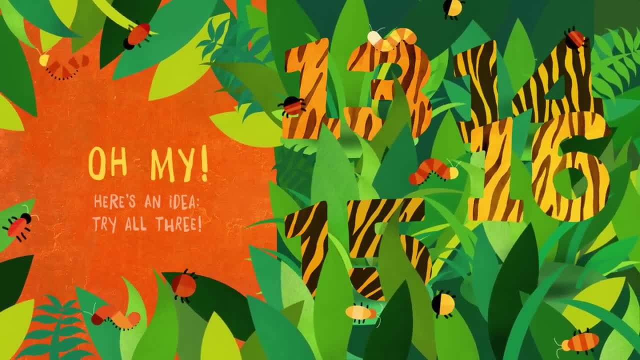 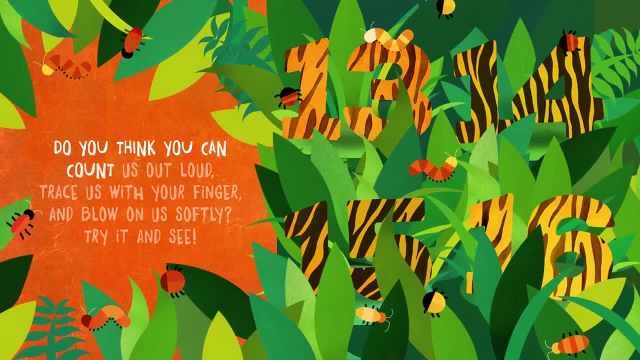 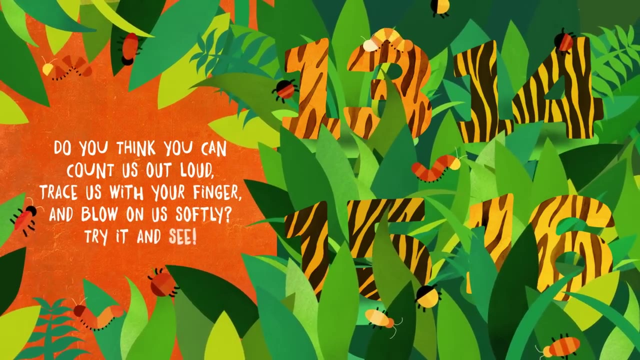 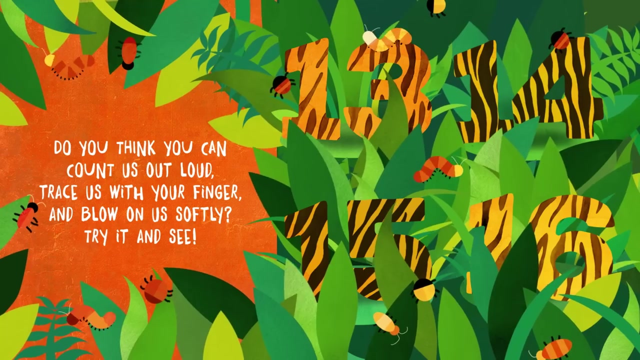 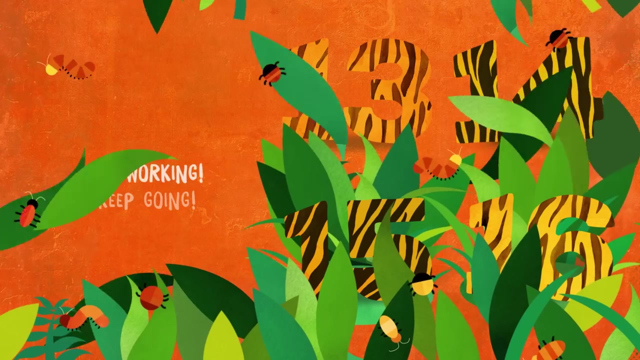 Oh, my, Here's an idea. Try all three. Do you think you can count us out loud? trace us with your finger and blow on us softly? Try it and see: Thirteen, Fourteen. It's working, Keep going. 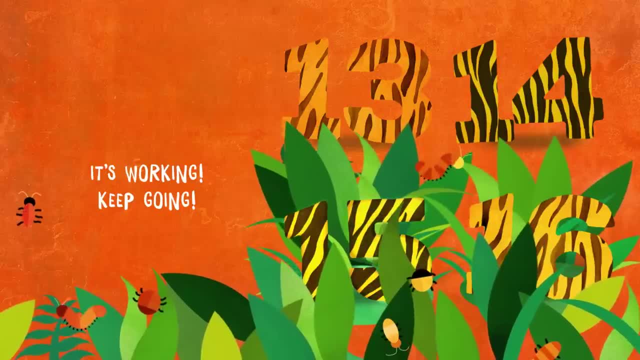 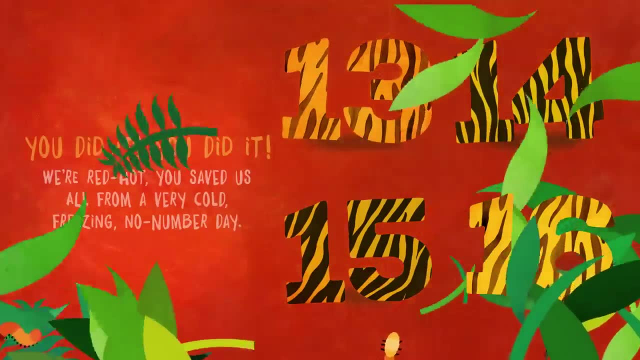 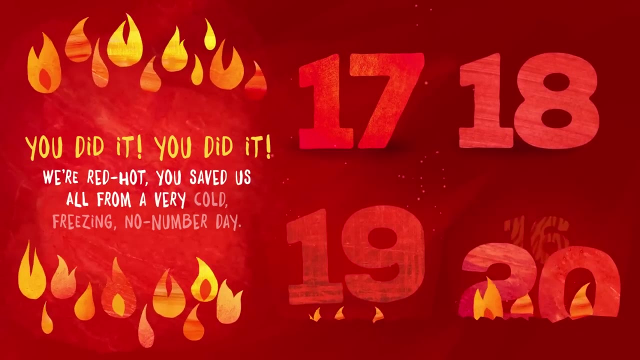 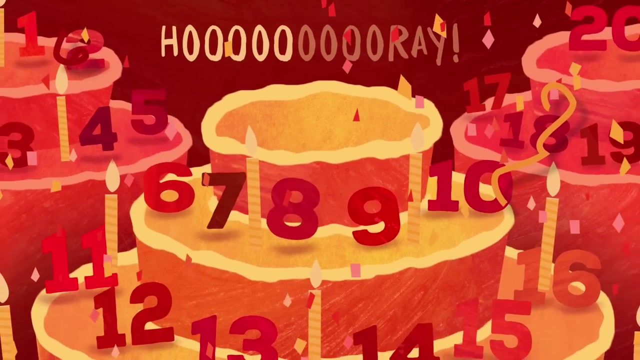 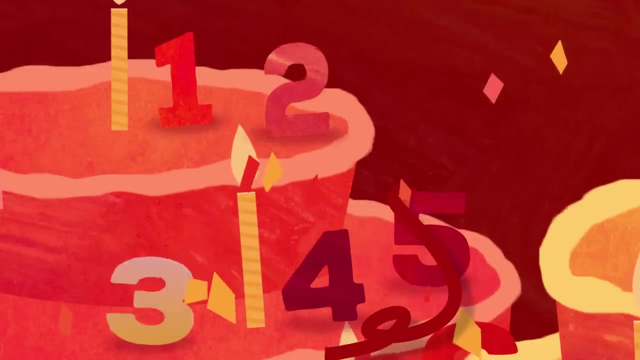 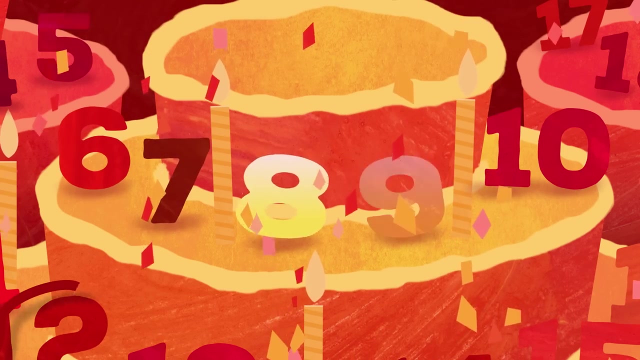 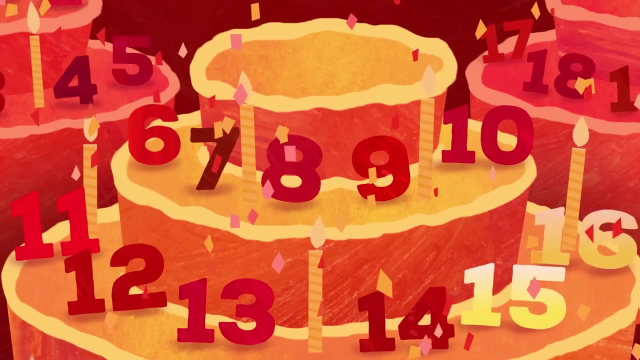 Fifteen, Sixteen, You did it, You did it, We're red-hot. You saved us all from a very cold, freezing no-number day. Hooray, One, Two, Three, Four, Five, Six, Seven, Eight, Nine, Ten, Eleven, Twelve, Thirteen, Fourteen, Fifteen, Sixteen, Seventeen, Eighteen, Nineteen, Twenty. 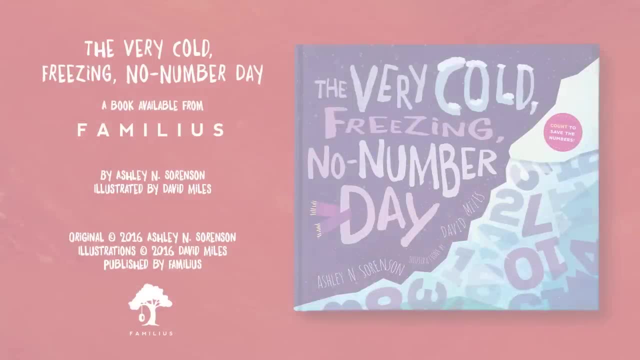 One, Two, Three, Fourteen, Sixteen, Seventeen, Fifteen, Eight, Nine, Ten, Eighty. Noah, you're done. You can't do anything. There's no one here. You're not talking to me. 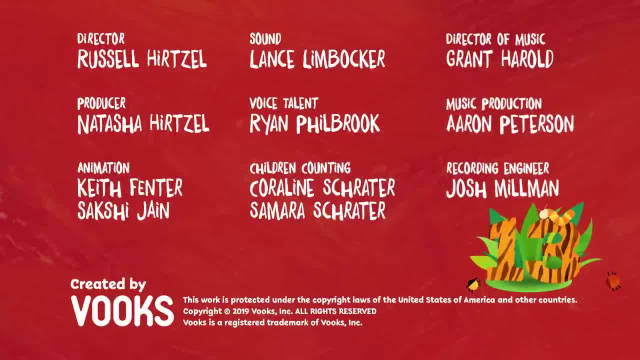 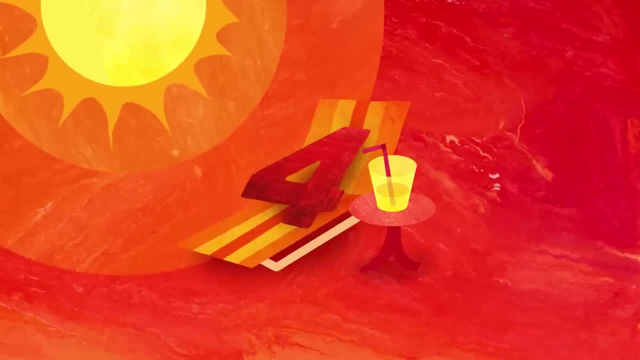 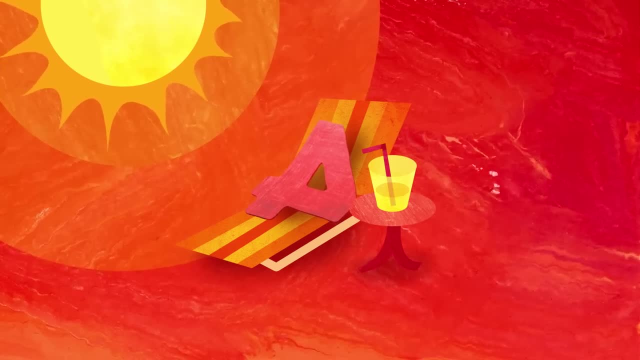 No, You're not talking to me. You're not talking to me. Oh Okay, One, Two, Three, Fourteen, Sixteen, Eighty, Nineteen, Sixteen, Eighty, Nineteen, Eighty, Nineteen, Eighteen, Decadent Seventy, Thirty, Forty Eighty, Sixteen Tens. 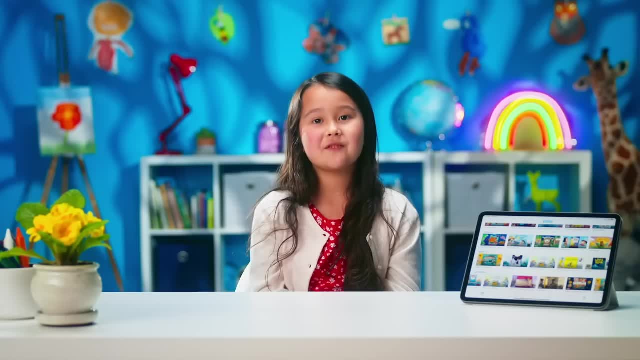 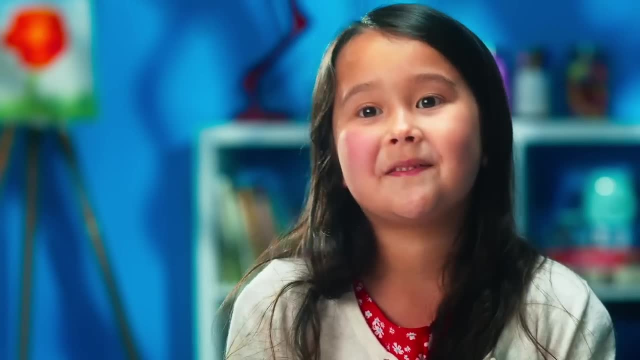 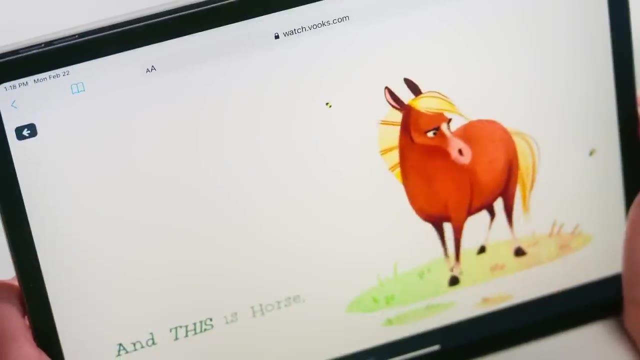 If you don't have books, what are you waiting for? It's a kid-safe, ad-free library full of storybooks brought to life. My favorite story on books is the Unicorn and Horse, because the horse feels like he's well, not beautiful, but he actually is. 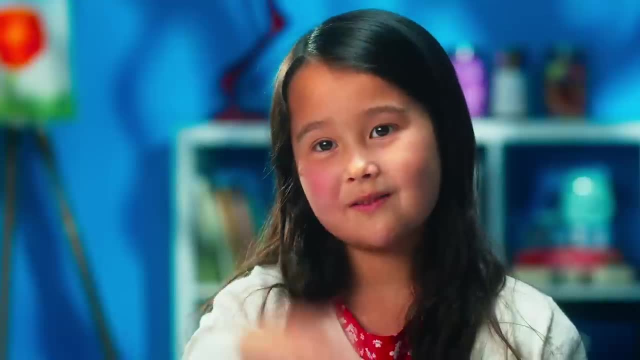 I'm going to explore more on books, and you should too. Don't wait around. Ask your grown-up and start exploring more fun stories like these. You'll be glad you did.